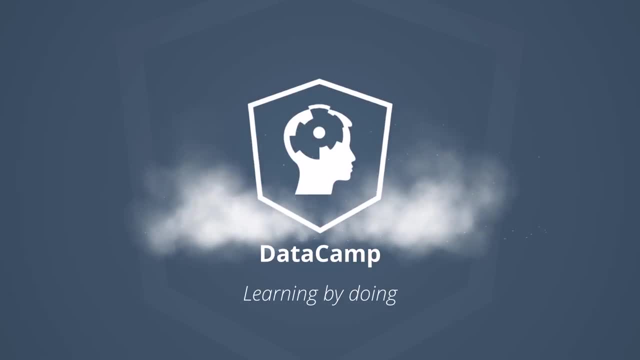 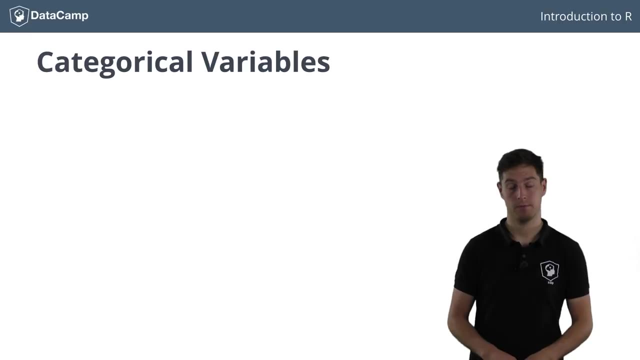 If you have some background in statistics, you'll have heard about categorical variables. Unlike numerical variables, categorical variables can only take up a limited number of different values. Otherwise put, a categorical variable can only belong to a limited number of categories. As R is statistical programming language, it's not a surprise that there exists a specific 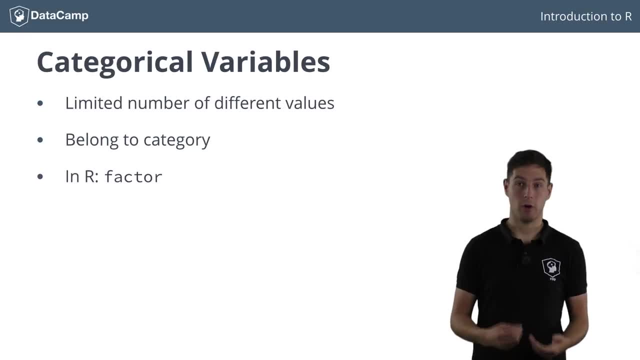 data structure for this the factor. If you store categorical data as factors, you can rest assured that all the statistical modeling techniques will handle such data correctly. A good example of a categorical variable is a person's blood type. It can be A, B, AB. 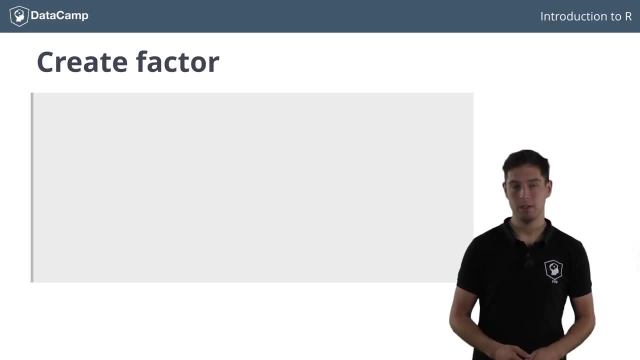 or O. Suppose you have asked 8 people what their blood type is and recorded the information as a vector blood. Now for R. it is not yet clear that you are dealing with categorical variables or factors here. To convert this vector to a factor, you can use the factor function. 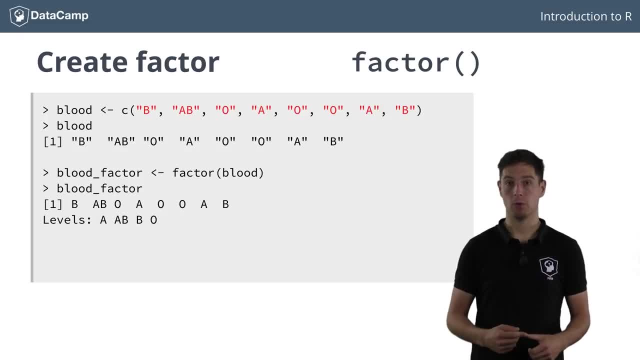 The printout looks somewhat different than the original one. There are no double quotes anymore and also the factor levels corresponding to the different categories are printed. R basically does two things when you call the factor function on a character vector. First of all, it scans through the vector to see the different categories that are in. 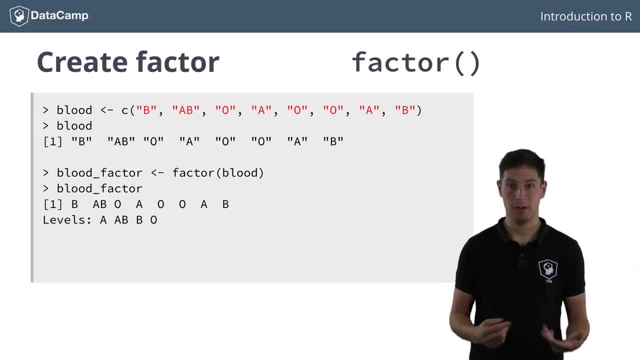 there. In this case, that's A, AB, B and O. It's here that R sorts the levels alphabetically. Next it converts the character vector- blood in this example- to a vector of integer values. These integers correspond to a set of character values to use when the factor is displayed. 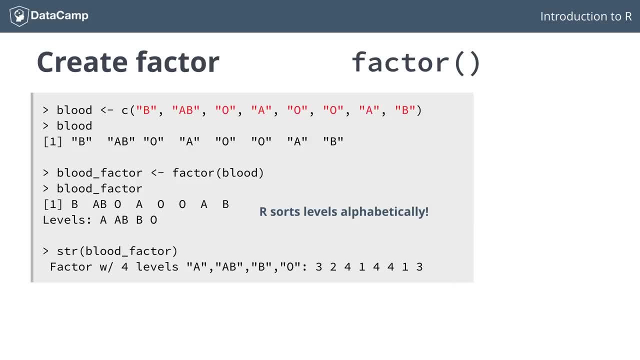 Inspecting the structure reveals this. We're dealing with a factor of four levels. The A's are encoded as 1, because it's the first level. AB is encoded as 2, B as 3 and O as 4.. But why this conversion? Well, 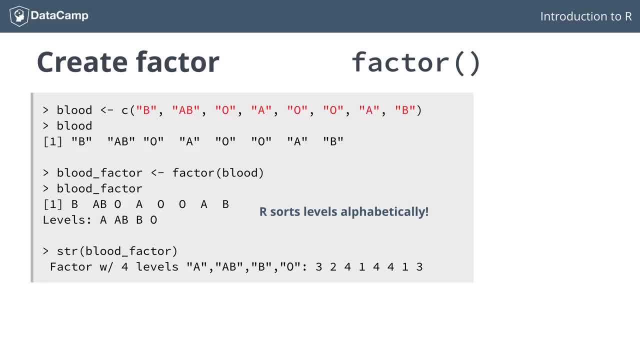 be that your categories are very long character strings Each time repeating the string per observation can take up a lot of memory. By using this simple encoding, much less space is necessary. Just remember that factors are actually integer vectors, where each integer corresponds to a category or a level. 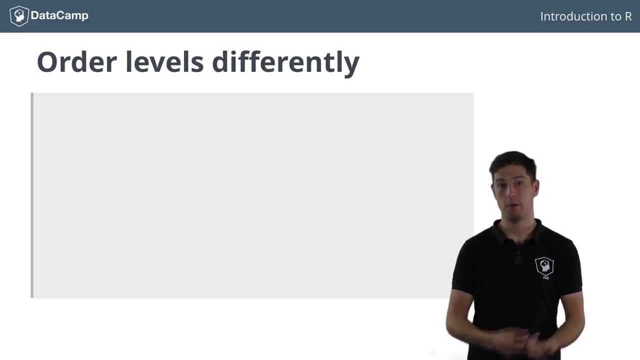 As I said before, R automatically infers the factor levels from the vector you pass it and orders them alphabetically. If you want a different order in the levels, you can specify the levels argument inside the factor function. If you compare the structures of blood factor and blood factor 2, you'll see that the encoding 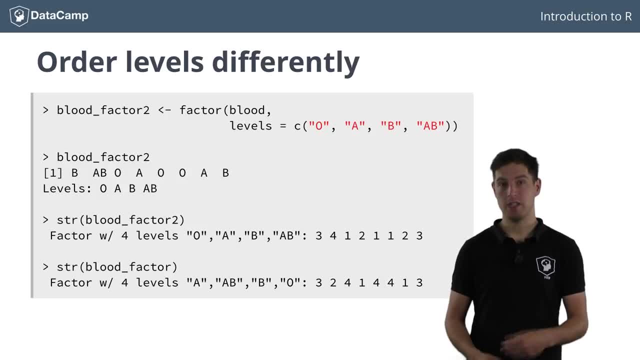 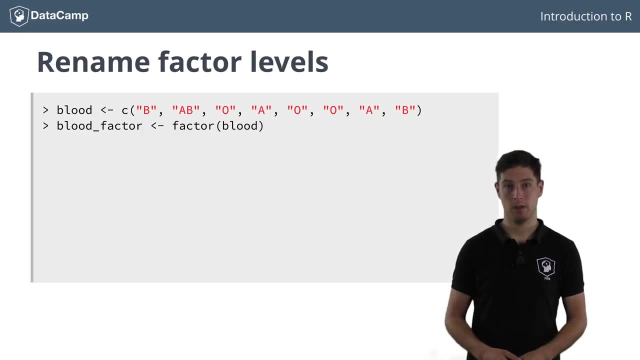 is different. now, Next to changing the order of the levels, it's possible to manually specify the level names instead of letting R choose them. Suppose that, for clarity, you want to display the blood types as BTA, BTAB, BTB and BTO. 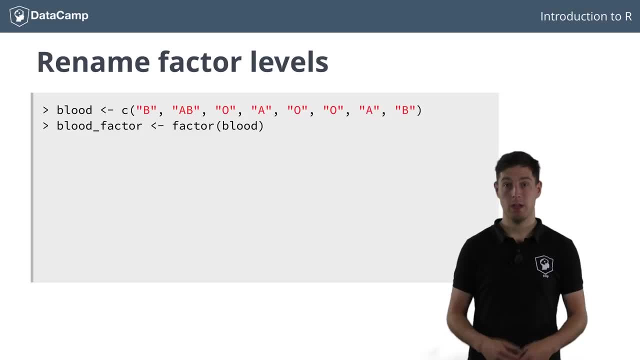 To name the factor afterwards. you want to display the blood types as BTA, BTAB, BTB and BTO. You can use the levels function, Similar to the names function, to name vectors. you can pass a vector to levels blood factor. 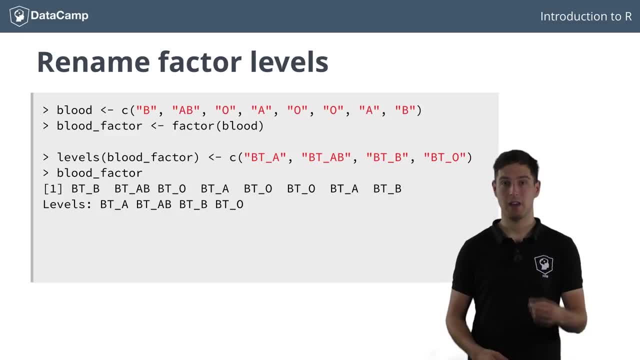 You can also specify the category names or levels by specifying the labels argument inside the factor function. I admit it, it's a bit confusing. For both of these approaches it's important to follow the same order as the order of the factor levels: first A, then AB, then B and then. 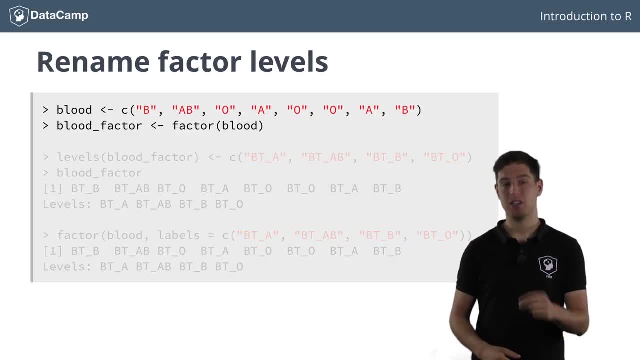 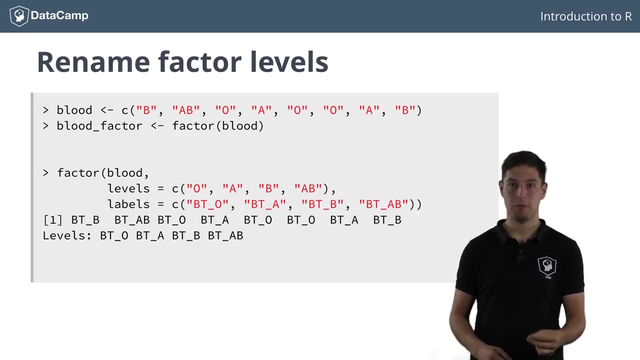 O. This can be pretty dangerous. You might have mistakenly changed the order. To solve for this, you can use the combination of manually specifying the levels and the label argument. when creating a factor With levels, you specify the order just like before, while with the labels you specify. 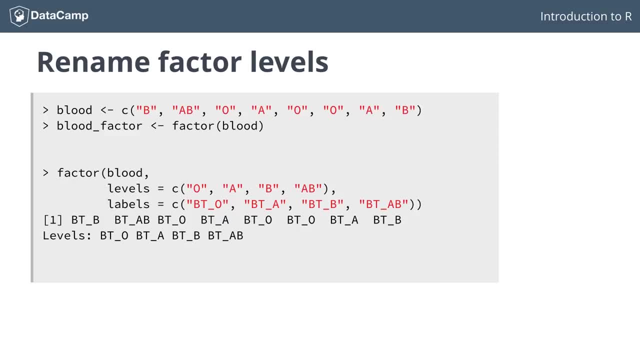 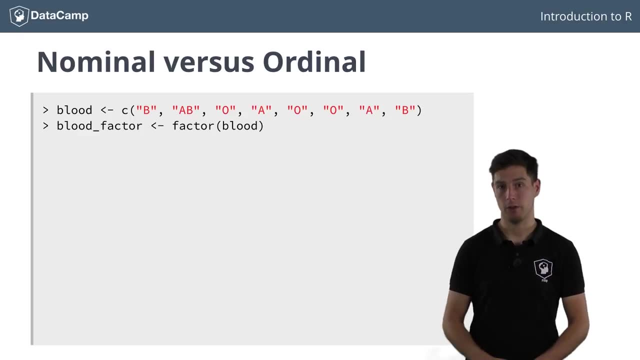 a new name for the categories. In the world of categorical variables there's also a difference between nominal categorical variables and ordinal categorical variables. categorical variables have no implied order. For example, you can't really say that the blood type O is greater or less than the blood type A. O is not worth more than A in any sense I can think of. 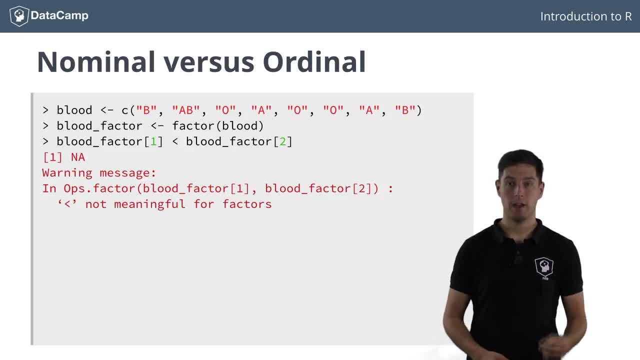 Trying such a comparison with factors will generate a warning telling you that less than is not meaningful. However, there are examples for which such a natural ordering does exist. Consider, for example, this t-shirt factor. It has codes ranging from small to large. 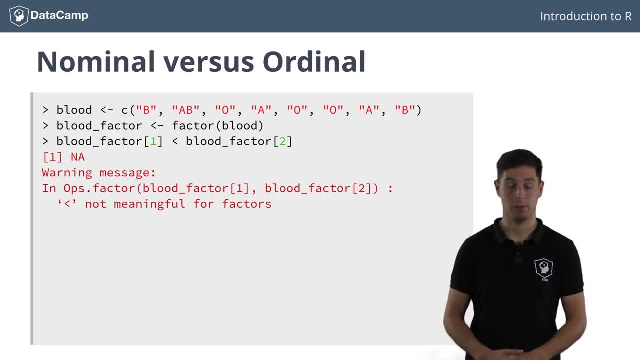 Here you could say that a large, indeed, is greater than a small, for example. right, Of course, R provides a way to impose this kind of order on a factor, thus making it an ordered factor. Inside the factor function, you simply set the argument ordered to true and specify the levels in ascending.